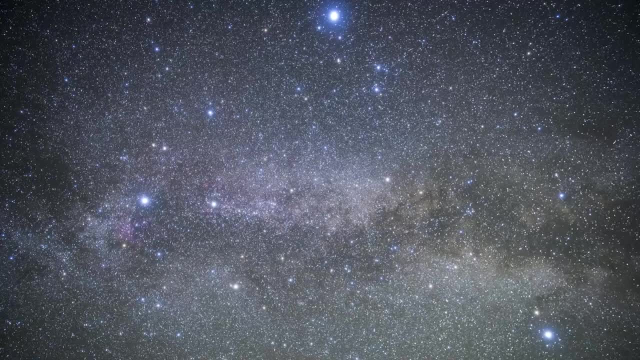 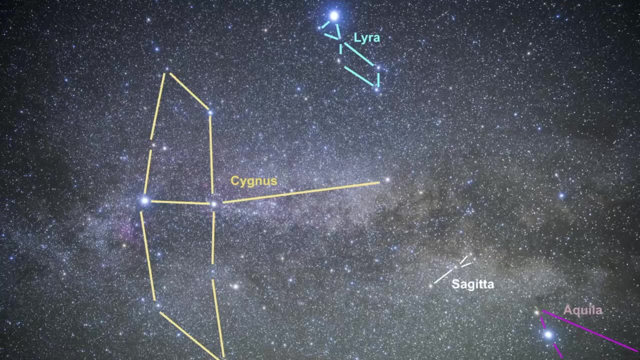 So G to the arrow constellation is fairly easy to find if you know where to look. It lies between Aquila and Cygnus, and the key to finding it is being able to identify the heads of both birds. You can also use the summer triangle asterism to aid you in locating this star pattern. 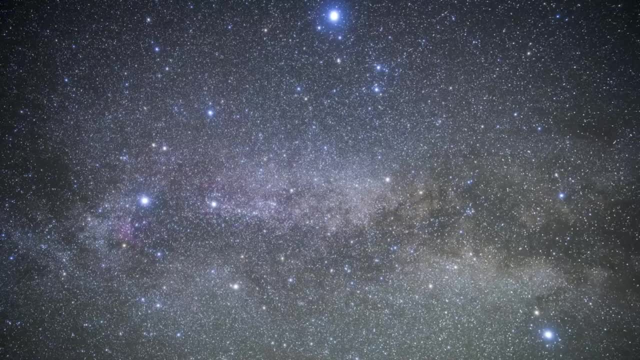 It is one of the smaller and less prominent constellations in the night sky, so to find it, seek out dark skies or use a stargazing app to help you. In this video, we will review how to find Sagitta, celestial objects to see in its borders and mythologies connected to this star. 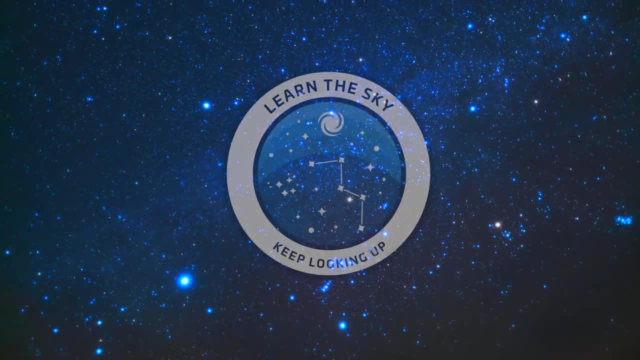 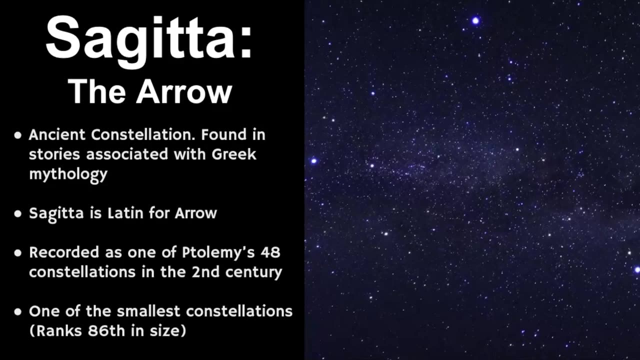 pattern. Welcome to Learn the Sky. My name is Janine and I'll be your guide as we explore the night sky, one constellation at a time. First, let's get a broad overview of Sagitta the Arrow. It is classified as an ancient constellation and it is connected with 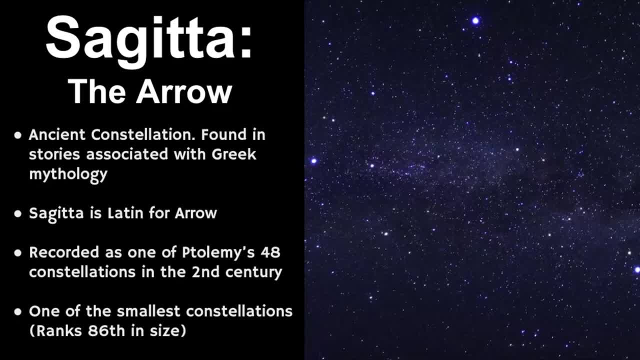 multiple stories found in Greek mythology. Its name is Latin for arrow and it was recorded as one of the most famous stories in the Greek mythology. It is also called Sagitta the Arrow, and it is one of the most famous stories in the Greek mythology. It is also called Sagitta the Arrow. 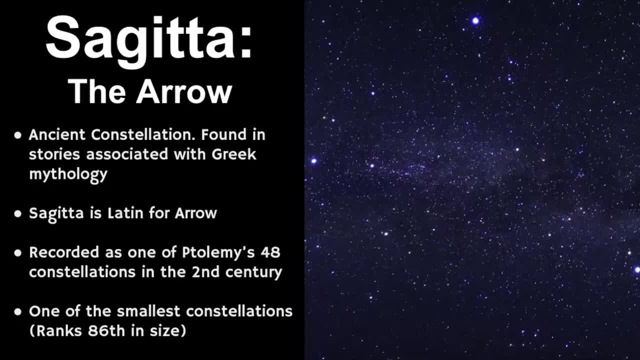 of Ptolemy's 48 constellations in the second century. It's one of the smaller constellations in the sky. It ranks 86th in size out of 88 constellations in total. So when can you go out? 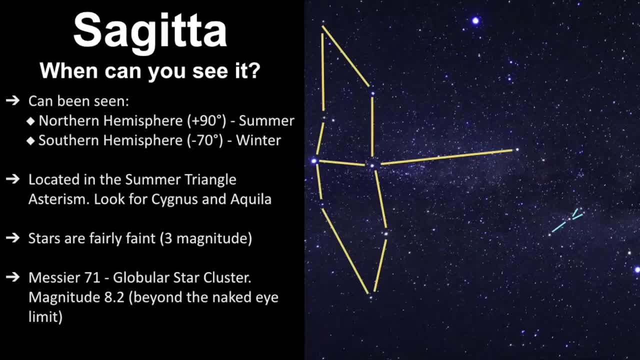 and see it. For people that live in the northern hemisphere, the summertime is the best time to look for Sagitta, But if you live in the southern hemisphere, you can see it pretty much everywhere, except probably Antarctica. This is the latitude in which you can see it at, from here to zero. 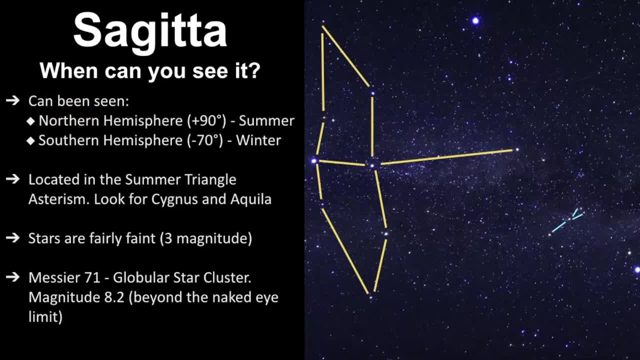 up to the equator, But there you have to see it in the wintertime because, remember, the seasons are opposite. The best way to find Sagitta is to look for the summer triangle asterism. I do have a whole video on that topic, so go see it for more information. But if you can identify the summer, 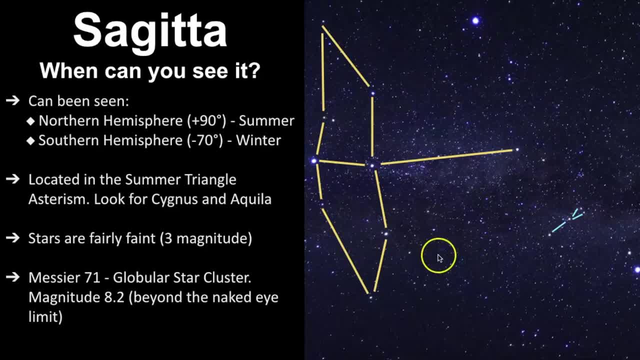 triangle you can find Cygnus, find the head of the swan, and Sagitta is nearby. Now the head of Cygnus is somewhat in this picture, but I've got some other practice photos for us to look at and explore so we can get practice finding Sagitta. The stars are fairly faint, so of third magnitude. 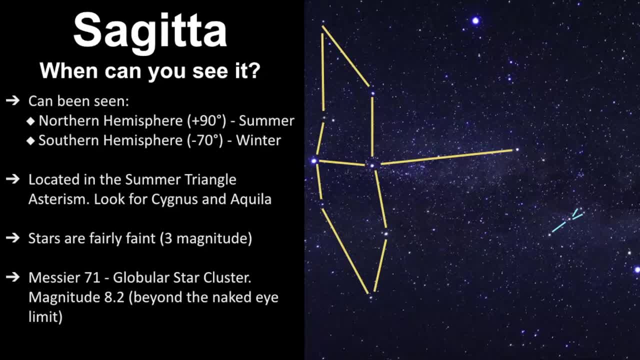 so it's best to seek out dark skies, And it is just a small constellation, so you need to get some practice with how to find it. In terms of celestial objects, there is a globular star cluster called Messier 71, but it is beyond the naked eye limit, so you would need 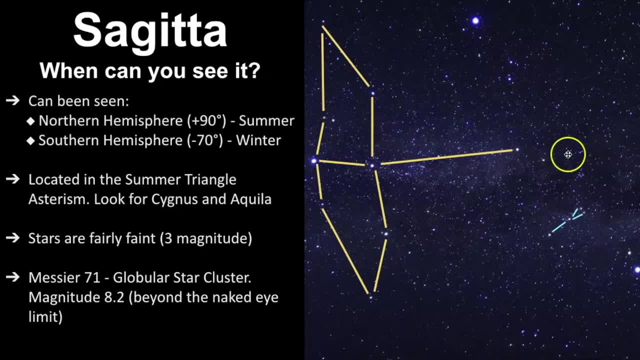 a telescope or binoculars to be able to see it. Right here is also the coat hanger asterism. It's not really located in Sagitta, but next door is Vulpecula the fox. but you can use Sagitta to. 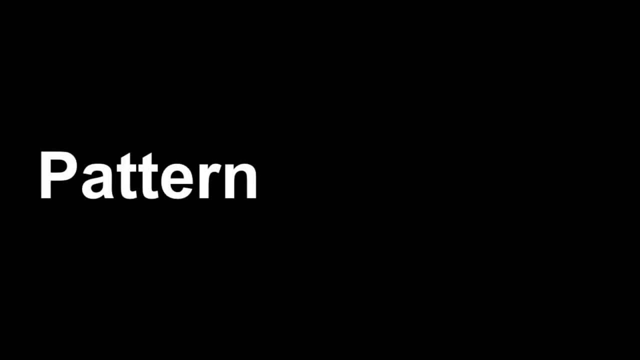 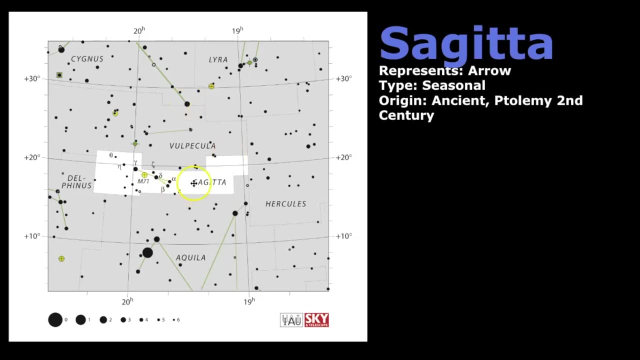 help you find the coat hanger: asterism. Now let's take a closer look at the pattern of Sagitta. So here we have the star map from the International Astronomical Union of the constellation known as Sagitta, and you can see that it is a very small constellation. 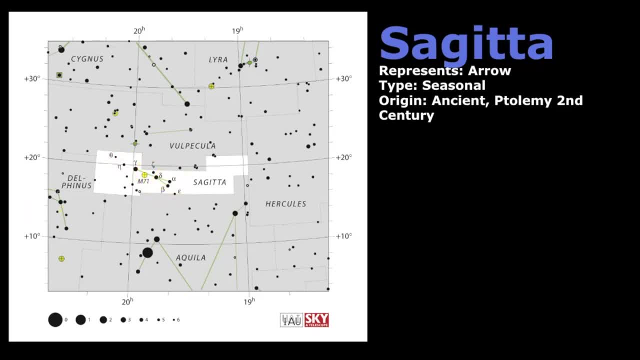 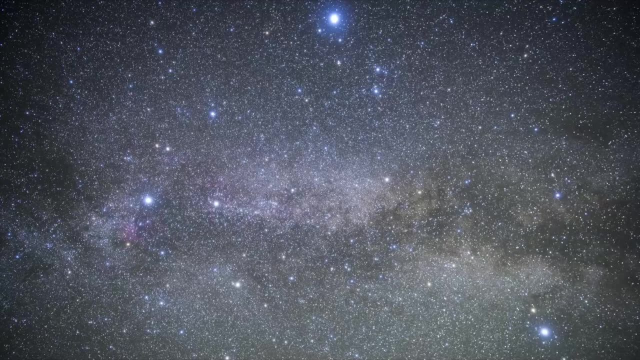 But its shape is distinctive and I can definitely see how it resembles an arrow. It is classified as an ancient constellation as well as a seasonal one, so you only can see it during certain times of the year. So let's get some practice looking at some pictures and how to identify it. This is: 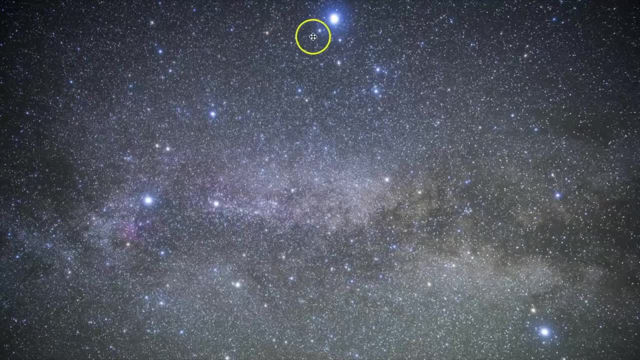 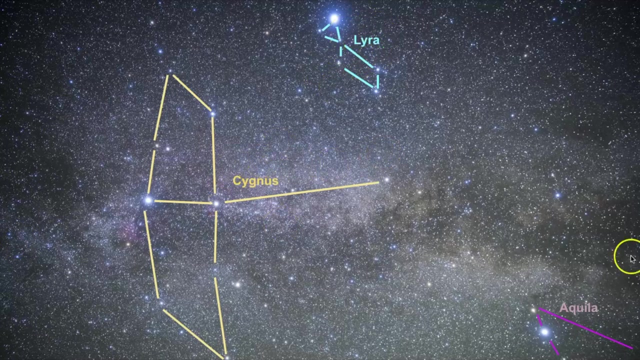 the original picture I showed you in the beginning of the video and hopefully your eye is drawn to the summer triangle right there and that's connected by the stars Vega, Neb and Altair. So here are the constellations: This is Cygnus, this is Lyra and this is Aquila. 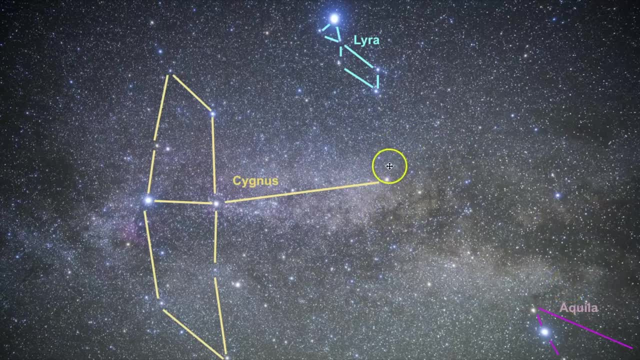 So, again, a trick for you to remember how to find Sagitta is: look for the heads of the birds. Cygnus is a swan, and this is where its head is located, and Aquila is an eagle, and here is where its head. 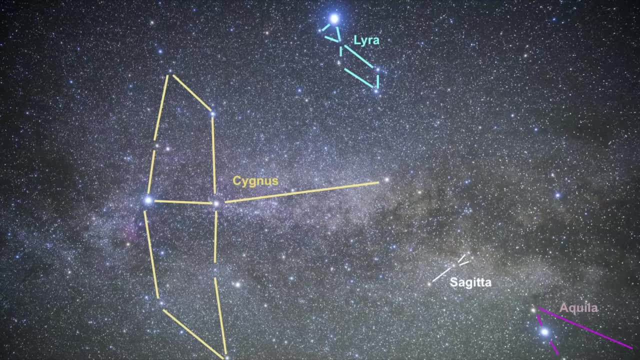 is located, And Sagitta is right in between the two. Now this is like a really great photo for you to look at. It's a long exposure photograph, so more stars are coming through. It's not quite realistic of what you would see in the night sky, but it's great to practice how to find it. 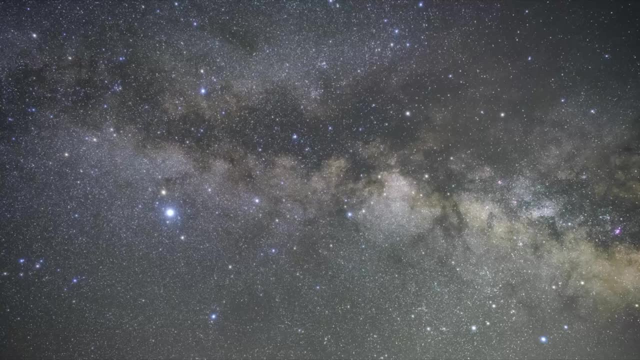 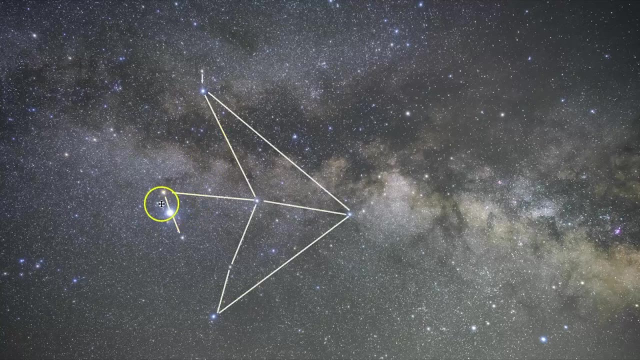 I've got a couple more photos for us to look at to help give us some practice finding Sagitta. So in this picture the main constellation is Aquila and you can tell because this star stands out. That star is Altair. I do have a whole video on that constellation and notice that the 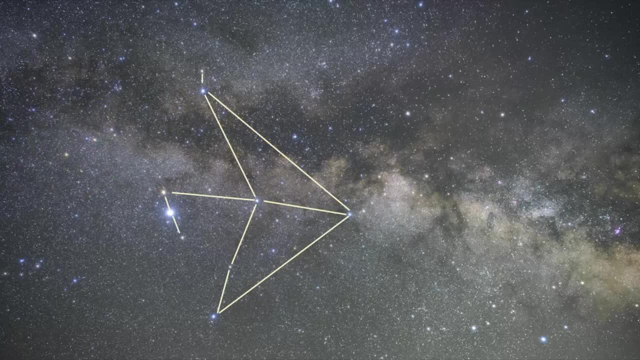 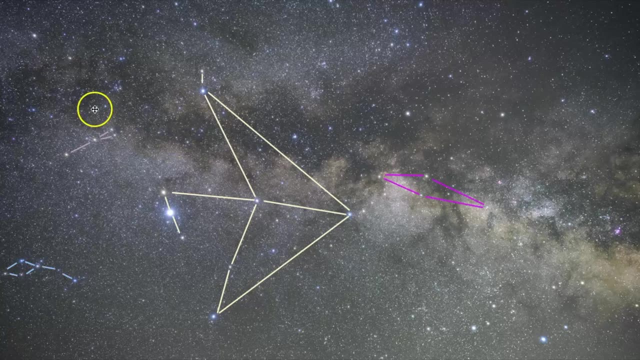 star is going through this entire photo and Sagitta is within the Milky Way as well. So here is where Scutum is and here are the other star patterns. You have Sagitta right here by the head of the eagle. This right here is Delphinus. I do have a video on these three. 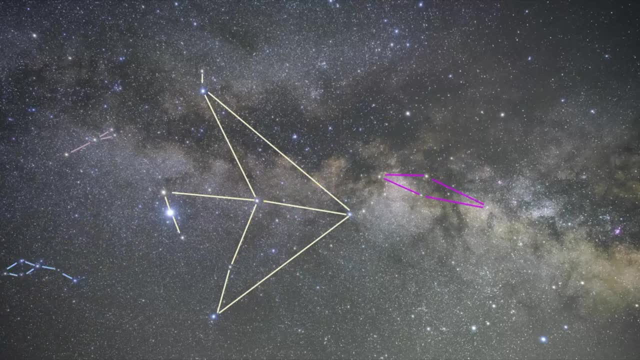 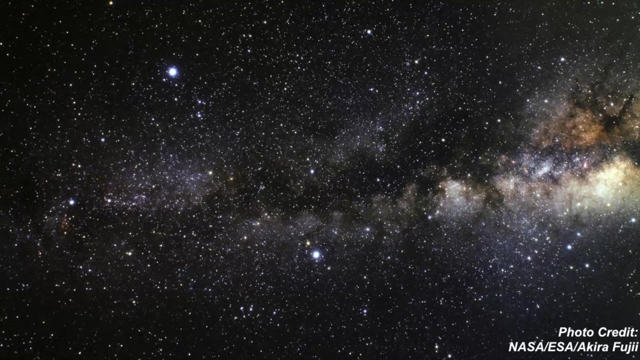 other constellations, so if you want to learn more about them, be sure to go see those videos. So again, another photo. This is a really good one. Here you can see the summer triangle. This again is a very high quality photo, but a little bit more realistic compared. 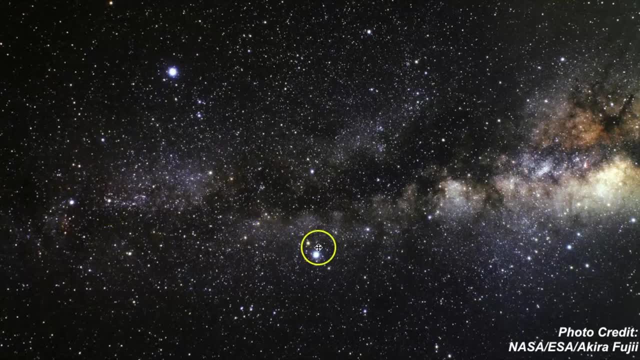 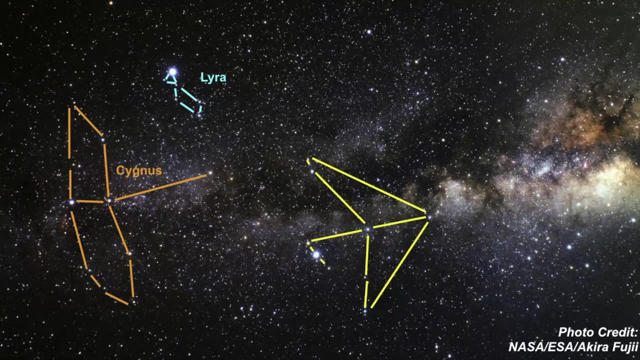 to the other two I showed you. So let's go ahead and find the summer triangle right there, and then from there you can find Aquila and the other constellations of Lyra and Cygnus, and then find the head of both birds right there and right there, And can you find Sagitta right? 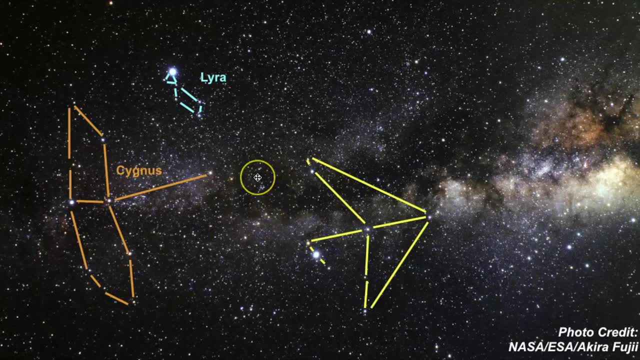 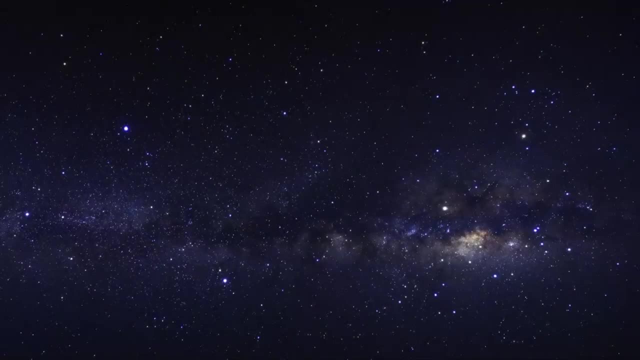 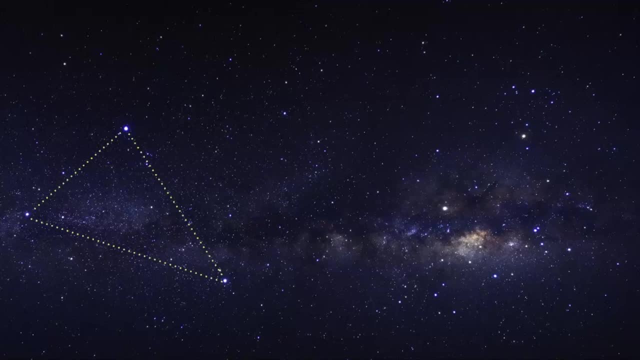 the photo Here is where it is, and then Sagitta is kind of towards the one angle of the triangle, the one that's closest to Aquila. So there it is, right there, and you can see it's not particularly bright, but its shape is distinctive. The constellations that are here are Aquila, and then we have 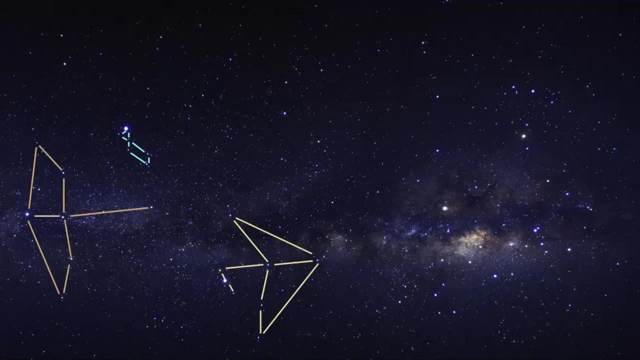 right here is Lyra, and then Cygnus, Some other constellations. to point out, This is where Sagitta is, This is Delphinus and this is Scutum, the shield. There is a lot going on here. Oh, I forgot. 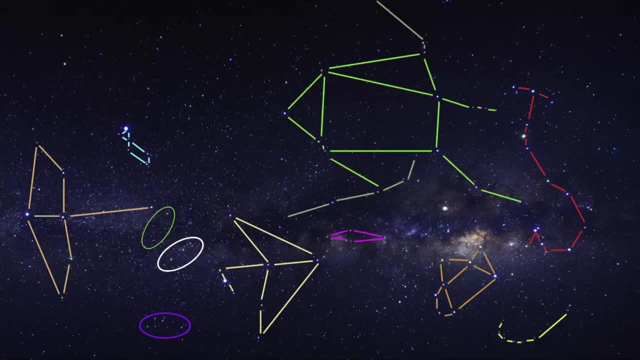 Vulpecula. There's a lot of other constellations here too, and just to point them all out, this is everything that you can see in the summer sky. Of course, this is a really great photo, so use it to kind of practice. You can pause. 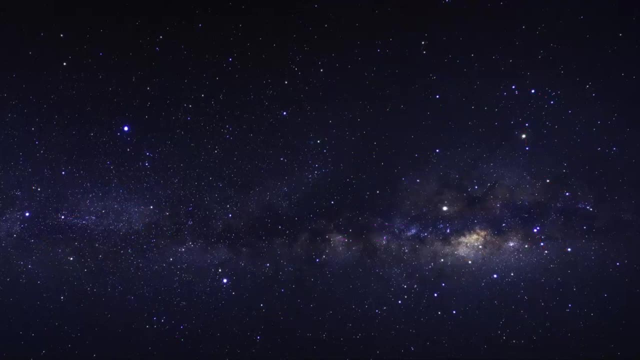 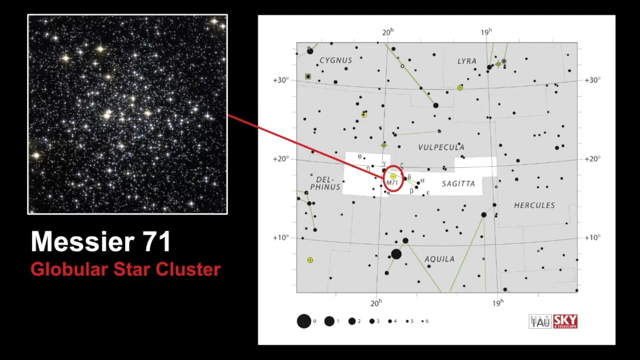 this video and go back and forth between these two photos to help give you some practice at identifying where things are and what is located to other constellations. Now let's take a look at some of the celestial objects that are located within the boundaries of Sagitta. Here we have the stellar map and notice how I circled Messier 71. This is a globular. 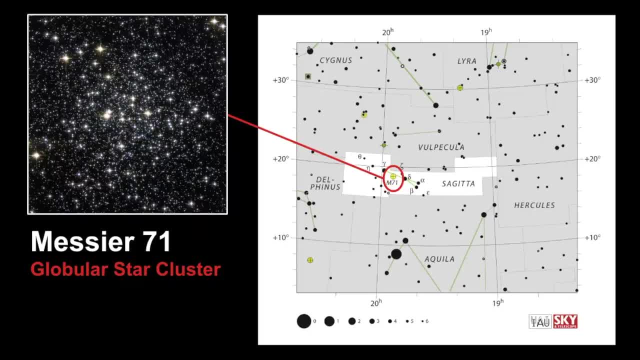 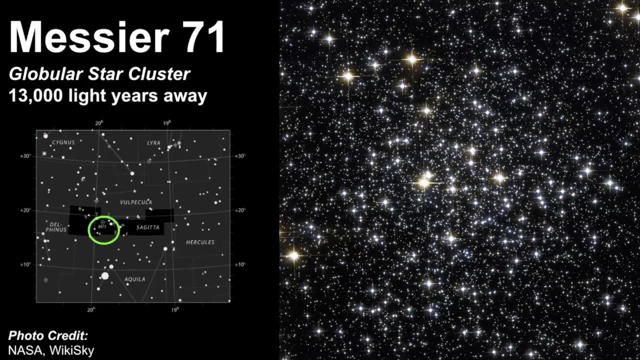 star cluster and it's underneath the naked eye limit, so you would need binoculars or a telescope to look at It. this is a beautiful picture that I found on nasagov, and this is such a beautiful star cluster. I have seen it through binoculars and it is fairly easy to point out because 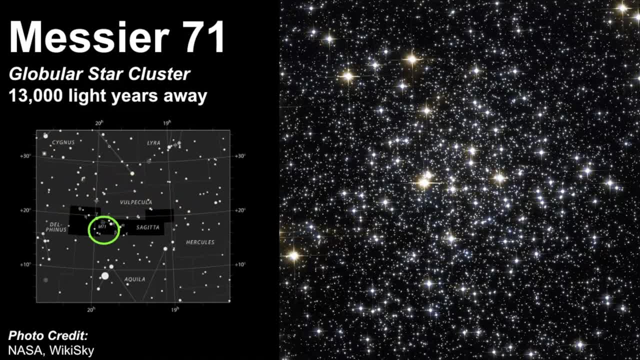 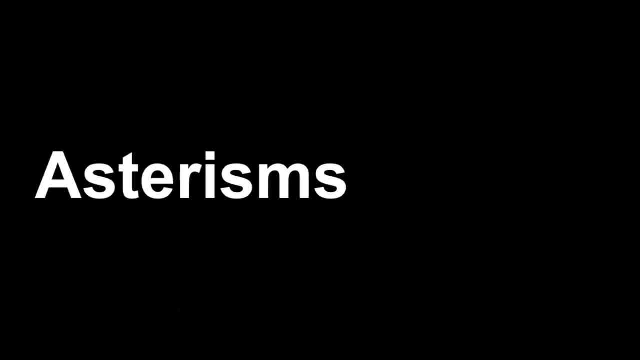 finding Sagitta truly is an easy thing to do when you have dark skies. This globular cluster is located 13,000 light years away, and don't forget about the asterism that is nearby. It's not necessarily located in Sagitta. 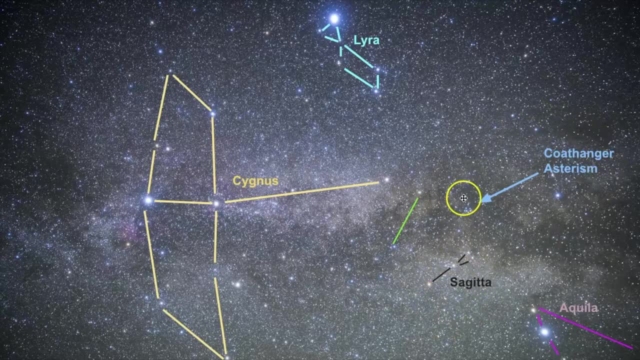 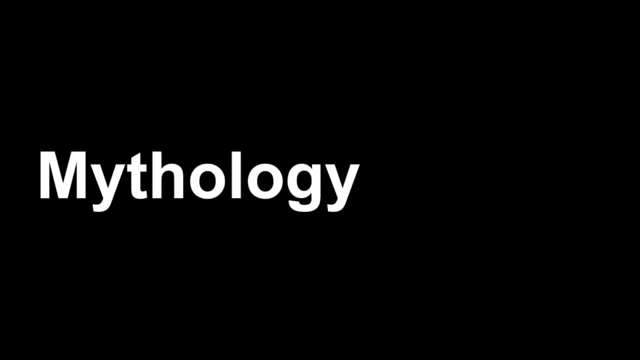 but the coat hanger asterism is very close to it, so use Sagitta to help you navigate and find the coat hanger asterism. Finally, we'll examine some of the legends that are connected with this constellation and keep in mind that there's no one true constellation story for any star pattern. 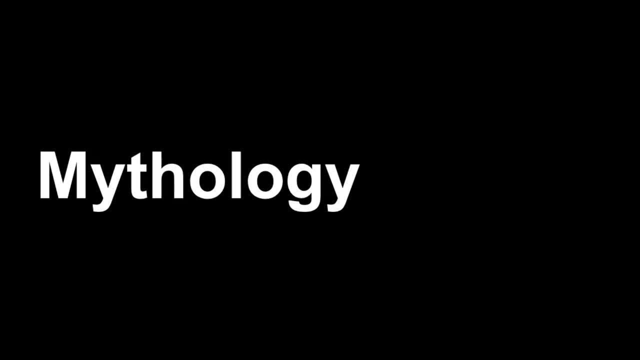 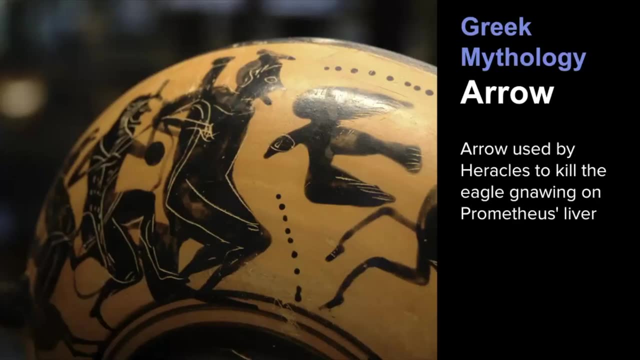 There's just a variety of legends that exist out there, depending upon the time and culture in which you are examining this legend, So for this video, I'm going to focus on Greek mythology. I found multiple stories that were connected to this constellation. One is the arrow used by 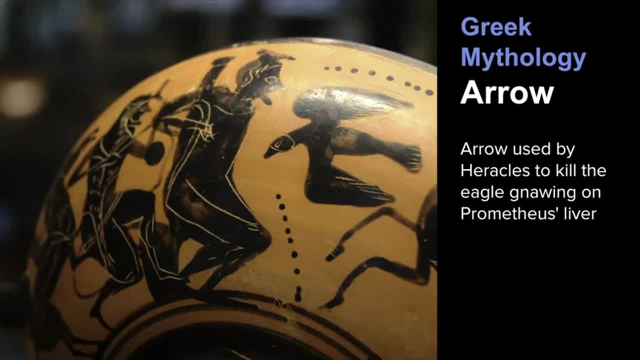 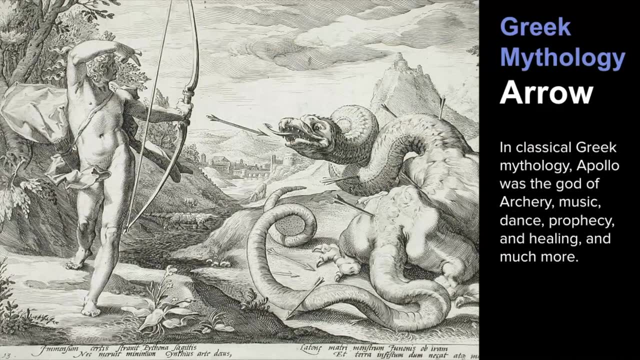 Heracles in Greek mythology that was used to kill the eagle that was gnawing on the liver of Prometheus. I also found another story about Apollo, and Apollo was the god of archery, music, dance, prophecy and healing and many other things, And here you can see an image of Apollo killing a python. 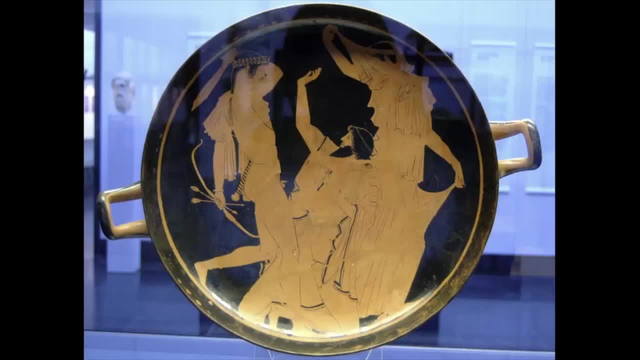 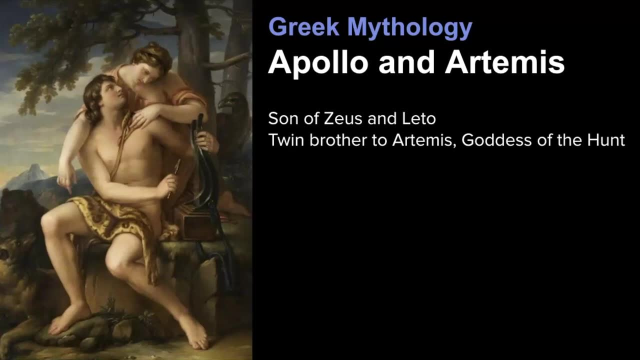 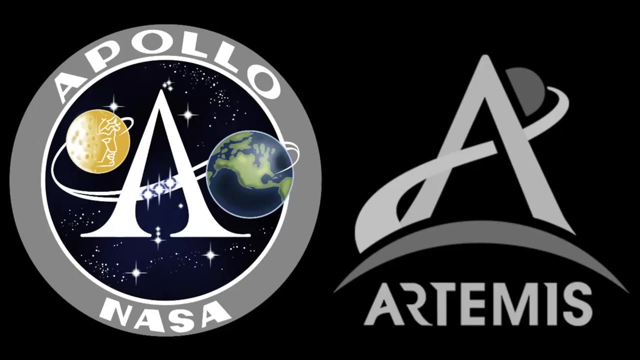 For those that are familiar with Greek mythology, when you think of Apollo, you probably often think of Artemis as well, because they are siblings and twins, for that matter, and Artemis is the goddess of the hunt. So as I was making this video, it made me think of these two NASA missions: The Apollo. 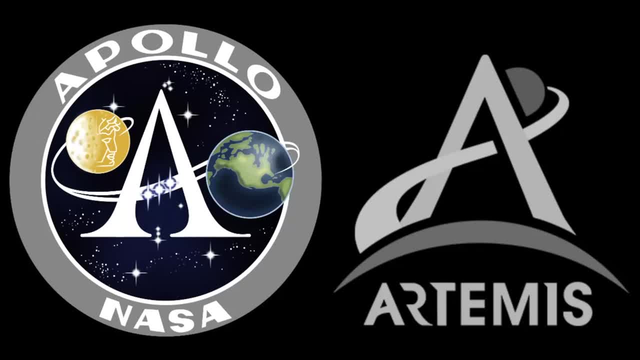 missions took place from 1960s and 70s, and it was all about orbiting the moon and landing astronauts there. The follow-up program to this in the current day is the Apollo mission. The first mission is Artemis, and that's about this is an international agreement between governments. 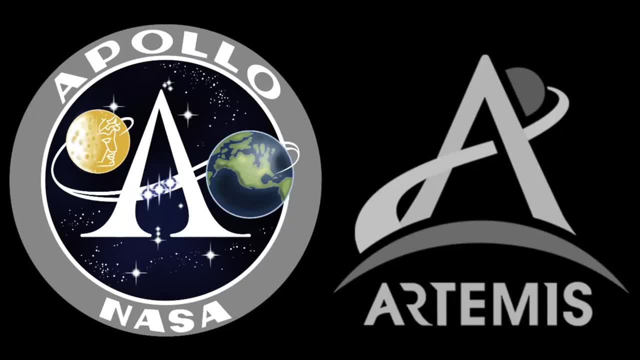 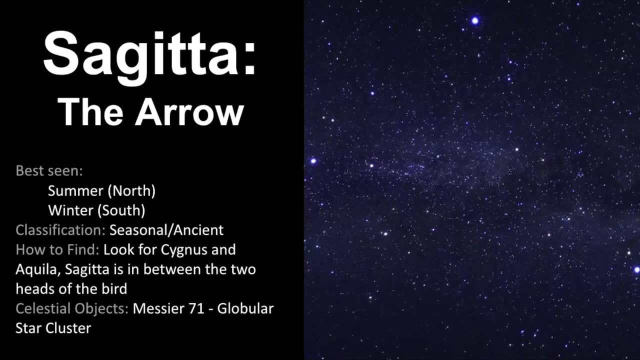 that in which NASA is leading the way, and this effort is to return humans to the moon by 2024.. And this will ultimately expand and deepen our space exploration adventures. We've come to the end of our video about Sagi to the Arrow, so let's review everything we've. 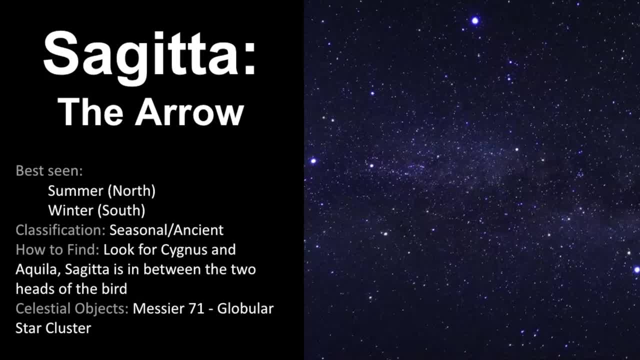 learned so far. It's best seen in the summertime in the northern hemisphere and in the wintertime in the southern hemisphere. What's nice is that it can be seen from both the northern and southern hemispheres, and it's classified as an ancient constellation as well as a seasonal one, so it's 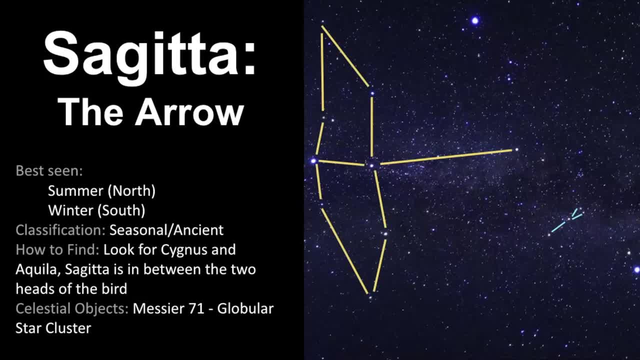 not one you can see all year round. The best way to find it is to look for Cygnus and Aquila, and Sagitta is in between those two constellations. The celestial objects that are located in it are Messier 71,, which is a globular star cluster, and then look for the asterism known as. 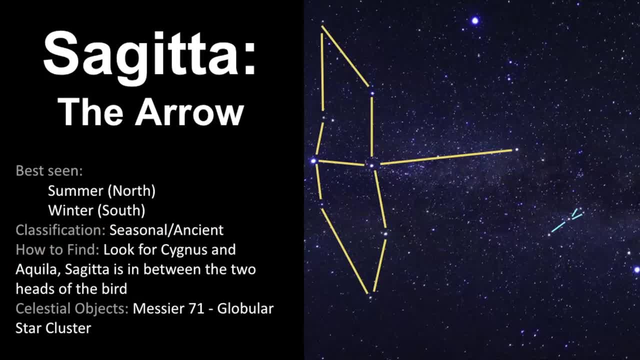 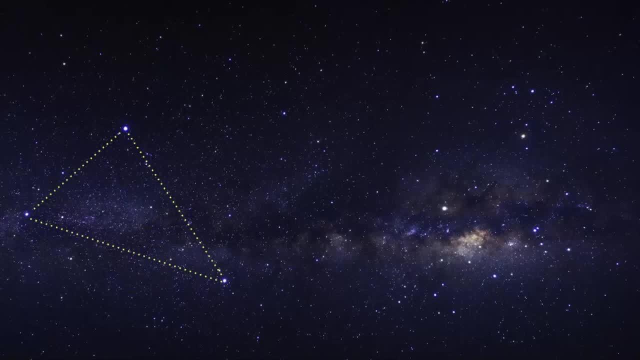 the coat hanger. I hope this video was helpful for you to hopefully find Sagitta. Remember, look for the summer triangle and then it is very easy to find, but of course I'm always going to recommend for you to go find dark skies. So thank you so much for watching. Let me know. 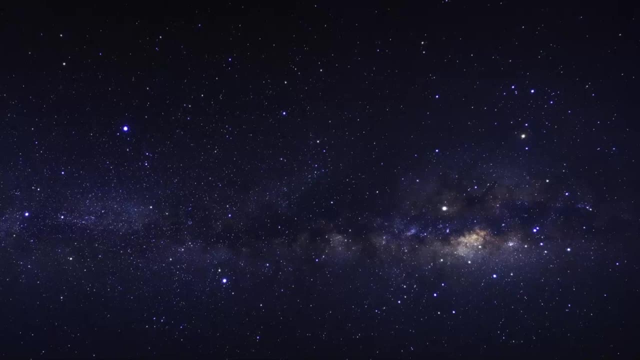 in the comments. have you seen this constellation And, if so, what was it like? Was it easy to find? Was it more difficult? And again, I always appreciate that you are here watching And for your positive feedback in the comments And if you have any questions. 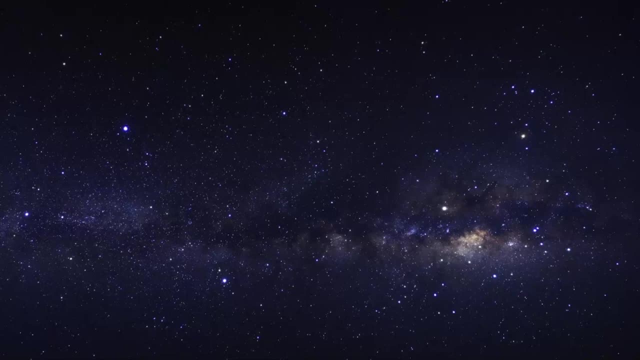 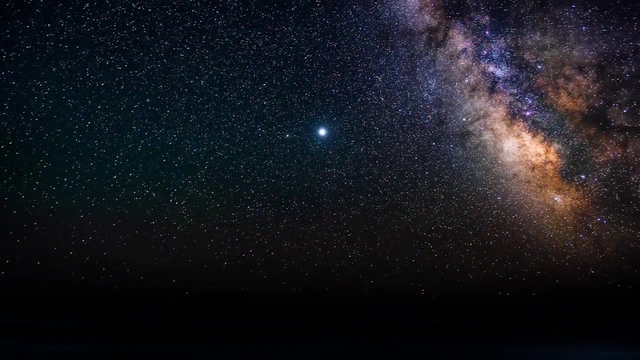 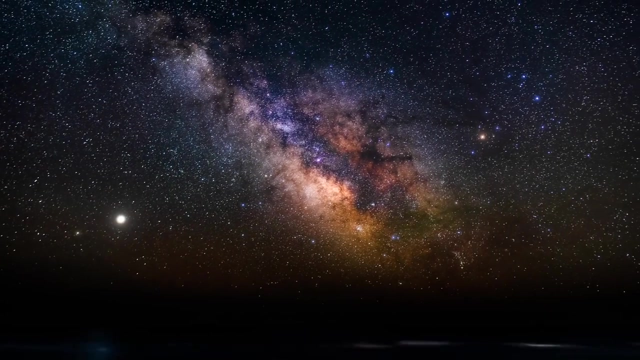 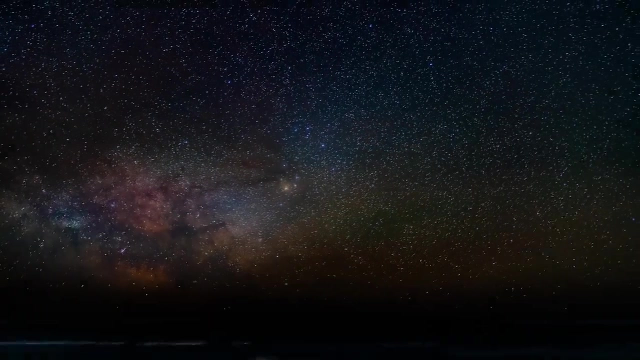 leave them in the comments below. And remember it takes time and patience to stargaze, So take a friend or a pet with you, go outside, take some time in nature and, as always, keep looking up. I'll see you in the next video. Bye, Bye.